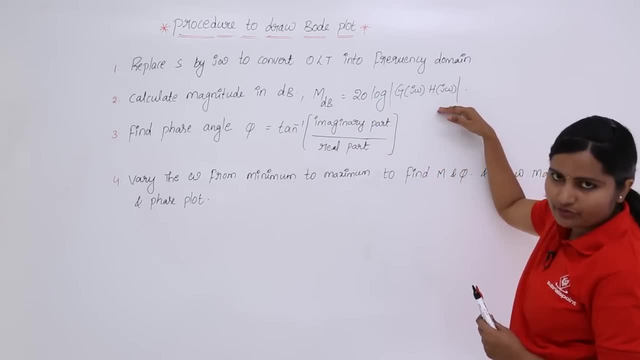 20 log more or less of g of j omega into h of j omega. So generally we are going to consider 20 feedback systems. So this h of j omega will be equivalent to 1. then we are going to consider 20 log. 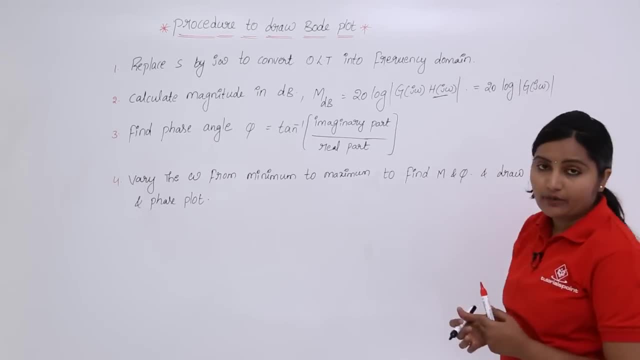 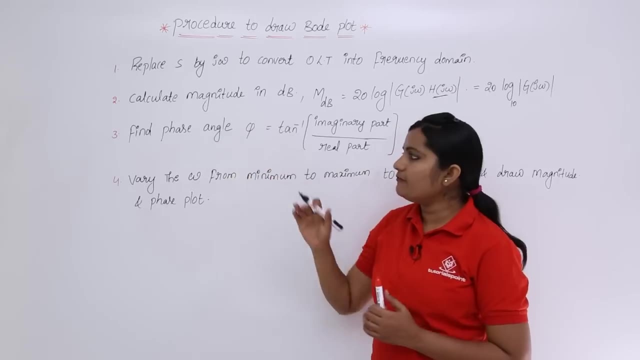 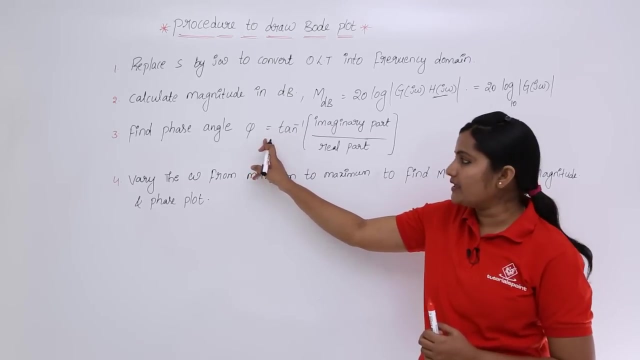 more or less of g, of j, omega. this will be the formula. So always, the base of this log is 10.. So now find phase angle phi. The next step is to calculate the phase angle. The formula to calculate phase angle phi that means, which is nothing but y axis of phase plot, is tan inverse. 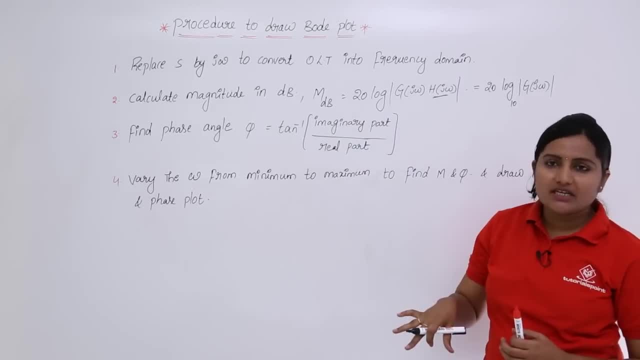 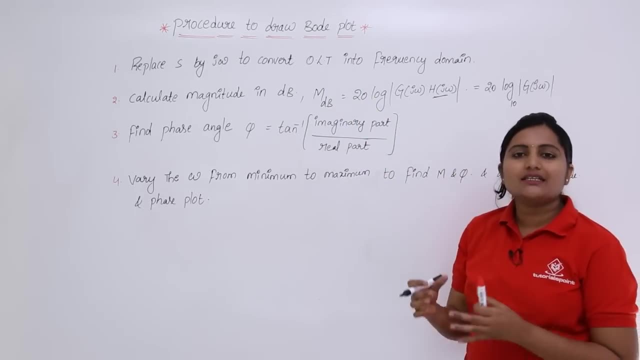 over T. So at y axis of phase plot is tan inverse of t. So you can calculate the time distance from the time distance And you can also work out the alpha axis. So for example, again this phi is equal to 1.. So that is 1 by 1. So this phi is equal. 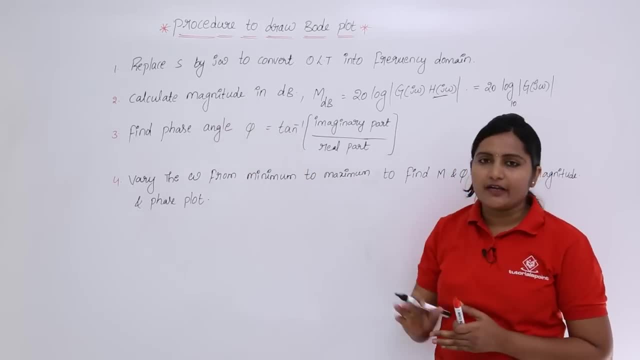 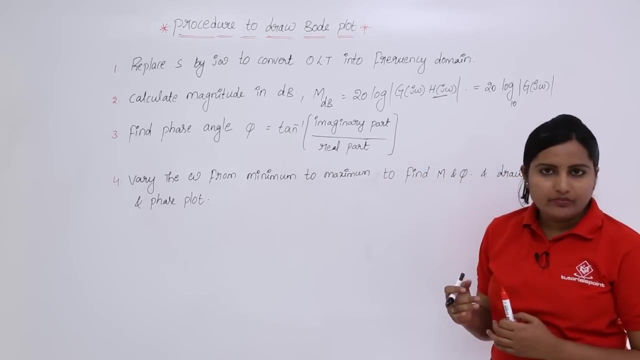 to 1 by 1.. Now this phi is equal to 1 by 1.. So we are going to get this phi. So you have to e to the power i. So this is the formula for e to the power i. So you have. 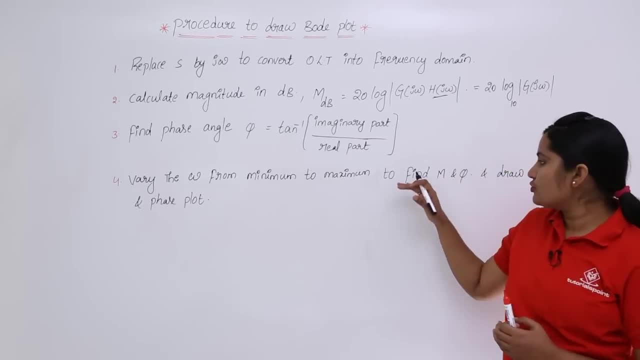 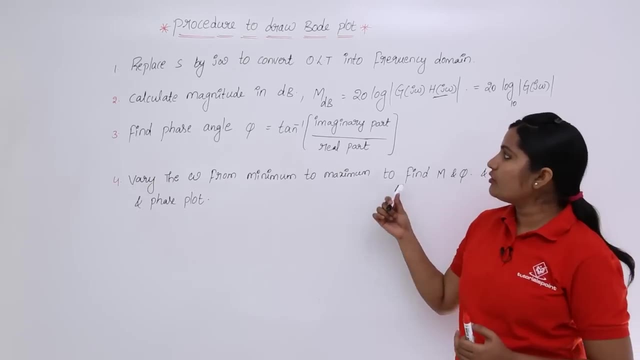 varying omega, from minimum to maximum, to find m and phi. you are going to get magnitude and phase plot, So you are going to calculate m in dB and after that phi. phi means tan, inverse, imaginary part by real part. So with varying omega, we are going to calculate that. 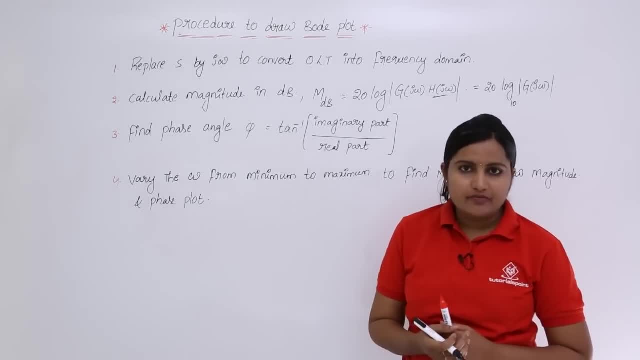 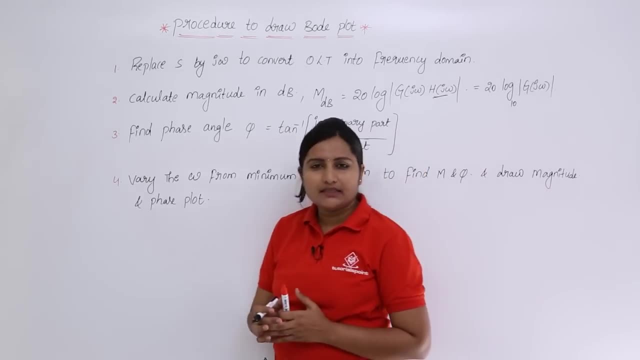 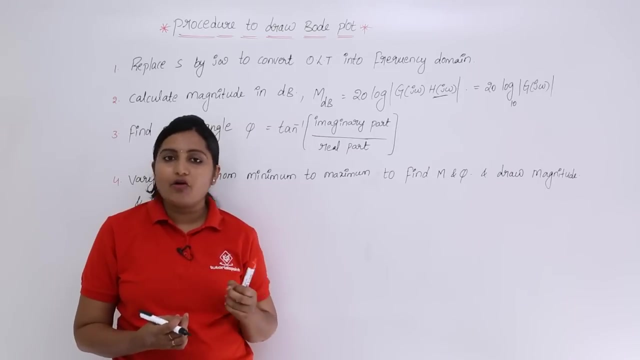 m and phi, and we are noting that in a graph. So then we are going to get magnitude and phase plots of our Bode plot. For example, in this video we already completed a list of basic Bode plots in that I given k, constant k, as our first Bode plot, So that also we 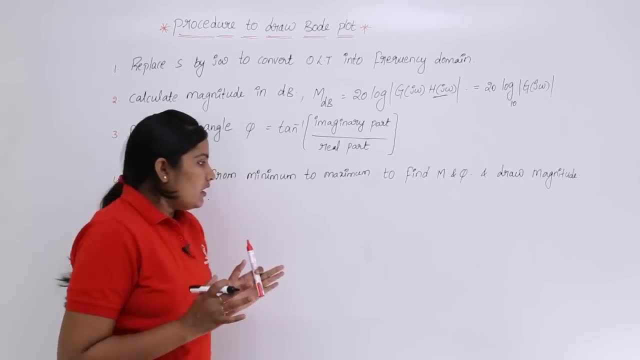 are going to cover in this video only. So here constant k means they given open loop transfer function. I am considering example. So here I am considering example of constant k. So here what is constant k means? This is the meaning: the open loop transfer function. 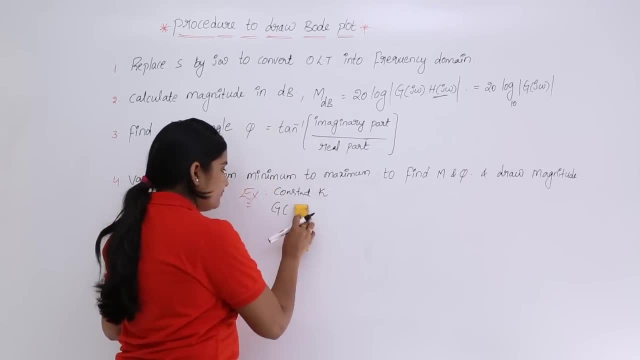 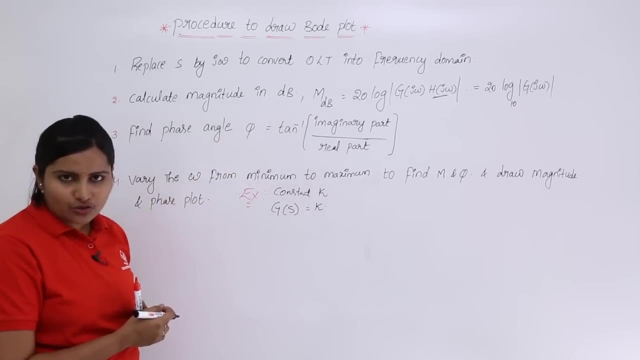 is equivalent to k. So, for example, if they given g of s is equivalent to k, if they given g of s is equivalent to k, then how will be the structure of Bode plot. So now we are going to calculate the structure of Bode plot. So now we are going to calculate. 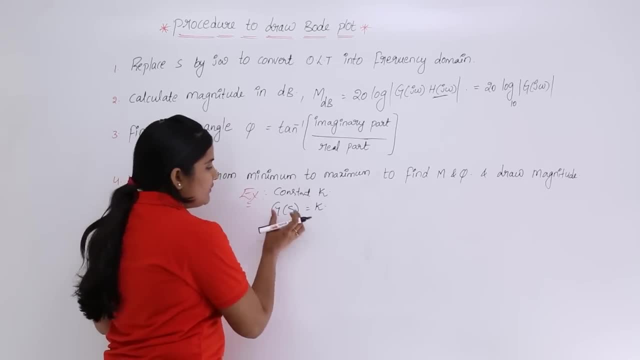 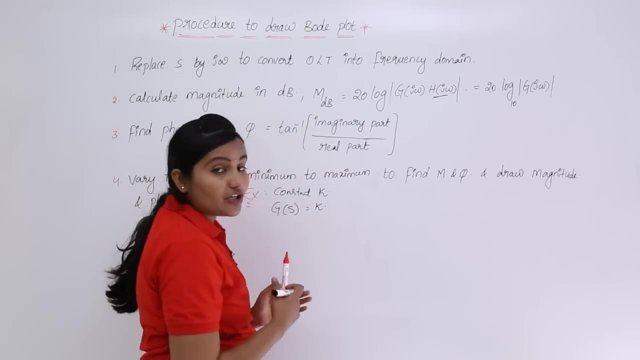 the structure of Bode plot. So now g of s is equivalent to k means. So, if you observe this, first step we need to do is we need to convert this open loop transfer function into frequency domain. How we can convert? Just by substituting: s is equivalent to j. 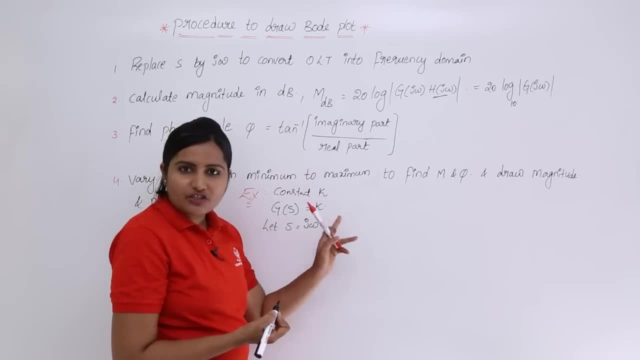 omega So we can convert this open loop transfer function into frequency domain. So here I am considering: s is equivalent to j omega. This side there is no s terms to substitute j omega. So here I am considering s is equivalent to j omega. So here I am considering, s is: 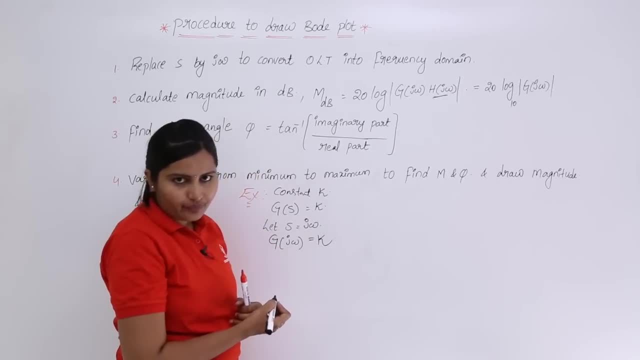 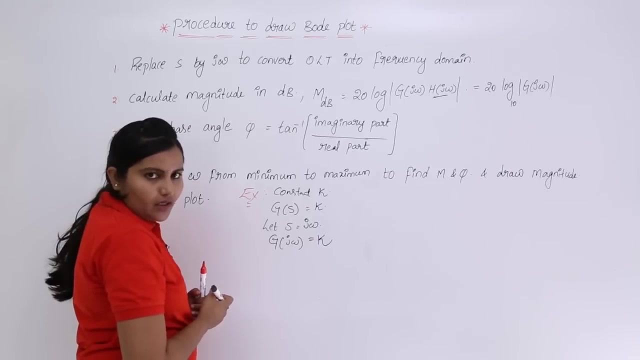 equivalent to j omega. So g of j omega also equivalent to k In other cases. for other terms, if you substituted j omega, whatever the s terms are there, that s terms are going to modify. So now, g of j omega is equivalent to k. So now, here, now I am going to calculate. 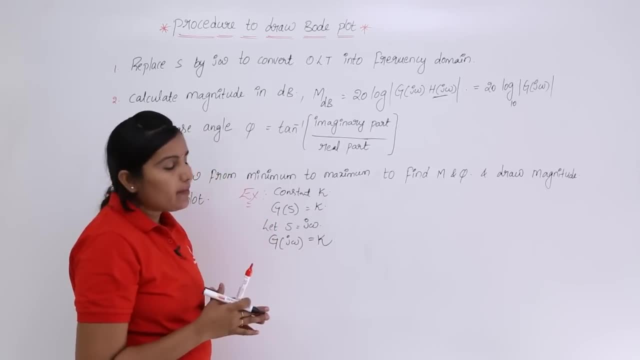 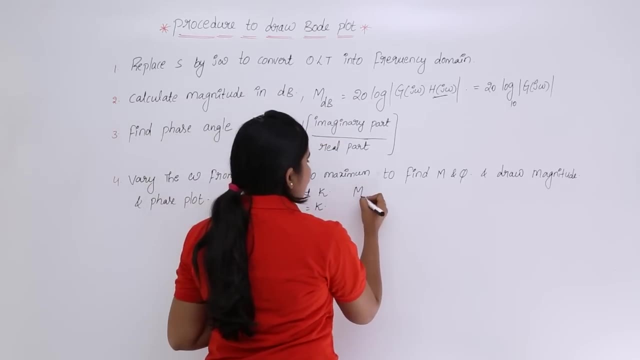 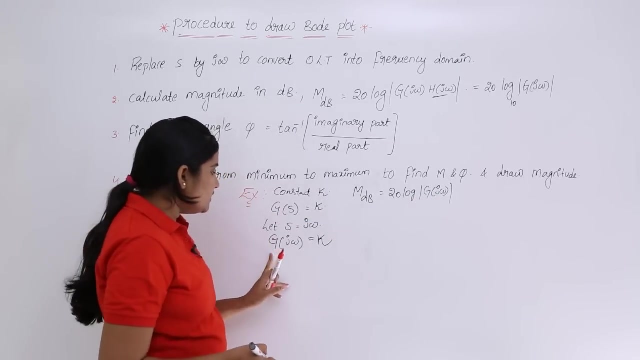 I am going to concentrate on magnitude plot. Magnitude plot means we need magnitude first of all. So magnitude In dB. m in dB is equivalent to 20 log g of j omega. h of j omega is always equivalent to 1, 20 log g of j omega. So here my g of j omega is equivalent to k. I am substituting. 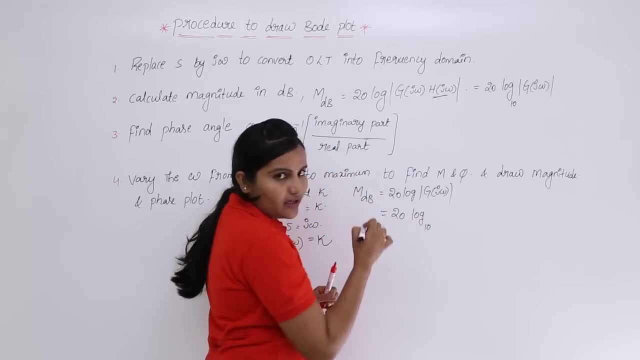 that 20, log base 10, always For this magnitude calculation. the log base is 10, and here modulus of g of j, omega 10.. The log base is 10, and here modulus of g of j, omega 10.. So here, 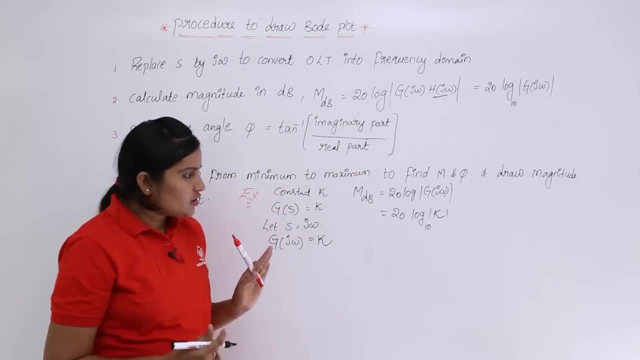 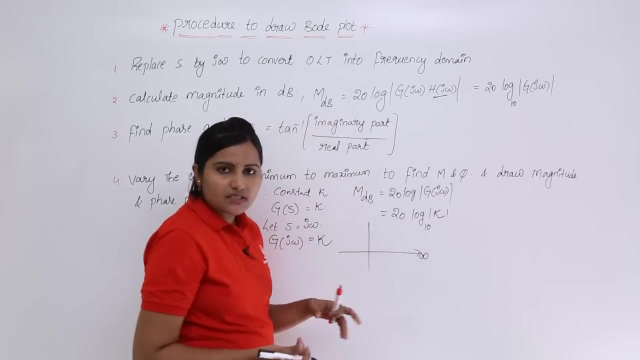 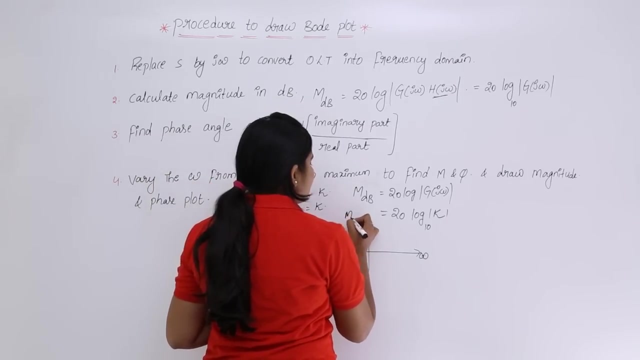 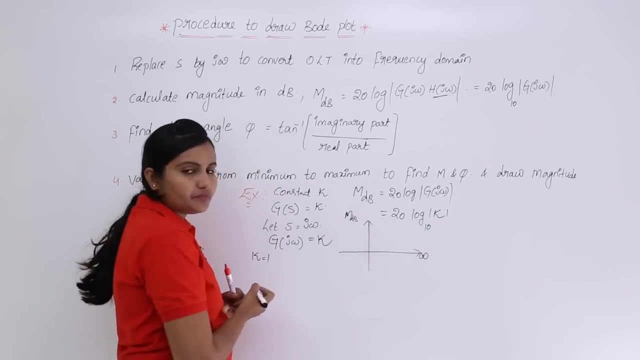 is nothing but modulus of k. So now, if you see this, depending upon the k value, the magnitude is going to vary. For example, this is omega, this is omega. x axis is always similar, this is omega. So this is magnitude in dB. For example, k is equivalent to 1, k is equivalent to 1.. What will? 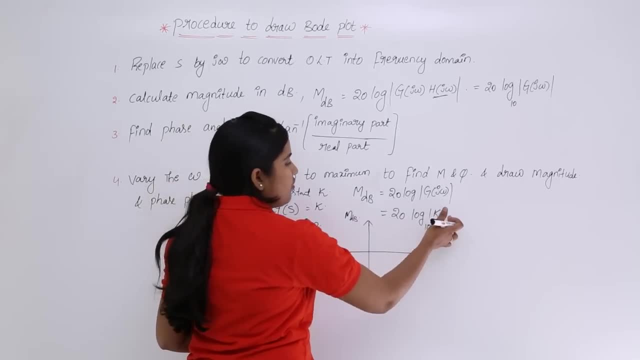 happens when k is equivalent to 1 means So this log 1 will be equivalent to 0. So then, when k is equivalent to 1, so you are getting like this: For example, k is greater than 1.. 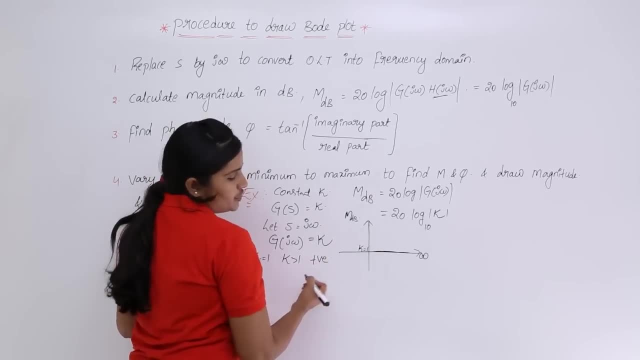 You will get positive magnitude. That means, if k is equivalent to 1, 2, that means greater than 1.. If k is greater than 1, means 2,, 3,, 4, 5, like that. then you are getting positive values. 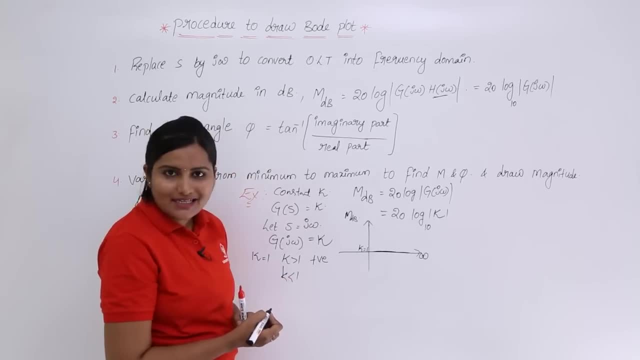 If k is less than 1, k is less than 1 means, for example, if you are given with k value like this, then you are getting positive magnitude. So you will get positive magnitude Like minus 2, minus 3, minus 4, like that or not minus. or if you consider 1 by 2, 1 by 3, 1 by 4. 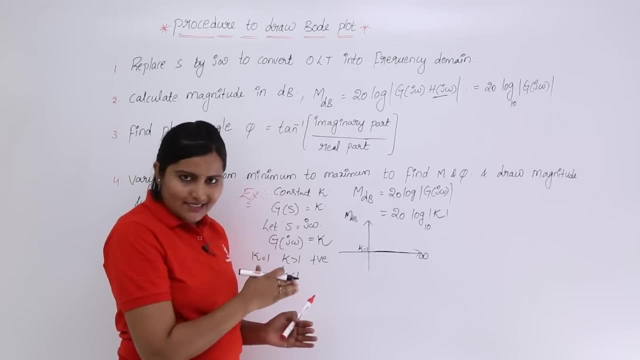 also equivalent to less than 1 case. That means less than k case, That means k less than 1.. So 0.5, also less than 1 case. minus 5, also less than 1 case. In all those cases, 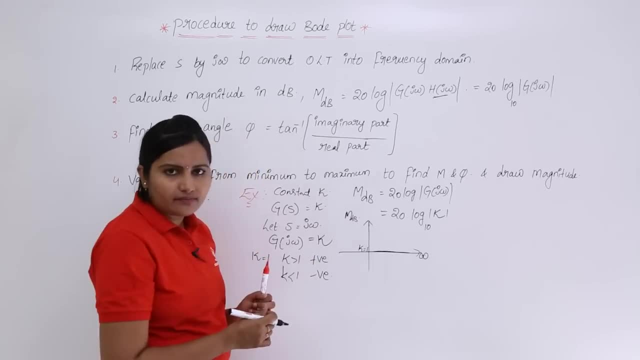 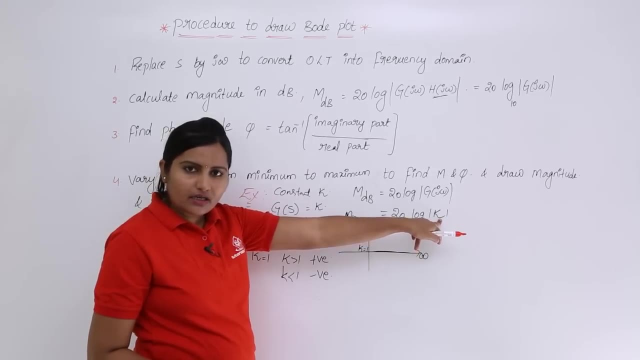 you are getting negative magnitude. You can check. For example, you just consider k is equivalent to minus 2 and you can consider calculation, you are going to get negative magnitude. If you consider k greater than 1 values, you are going to get all positive. 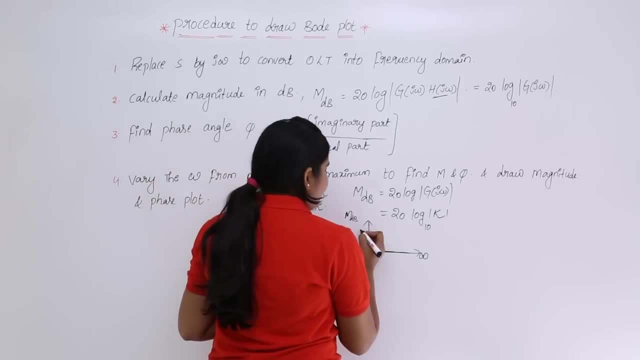 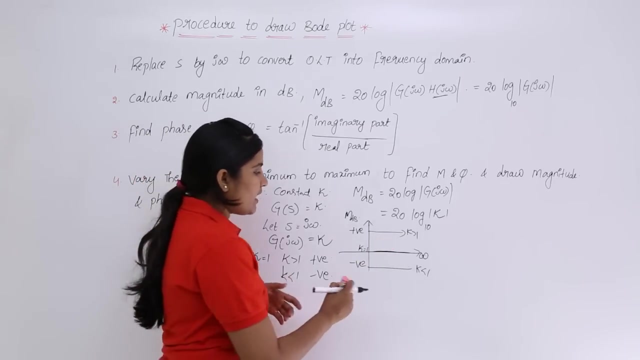 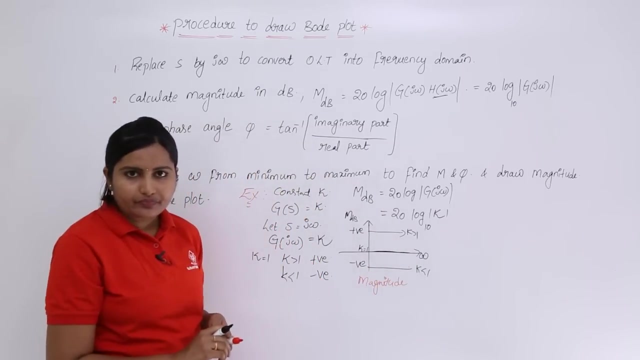 magnitude values. So here, if k is greater than 1, you are getting positive magnitude. 1k greater than 1.. When k less than 1, so you are getting negative magnitude. So this is your magnitude plot, This is your magnitude plot of constant k. Now coming to phase plot. So here, phase plot. 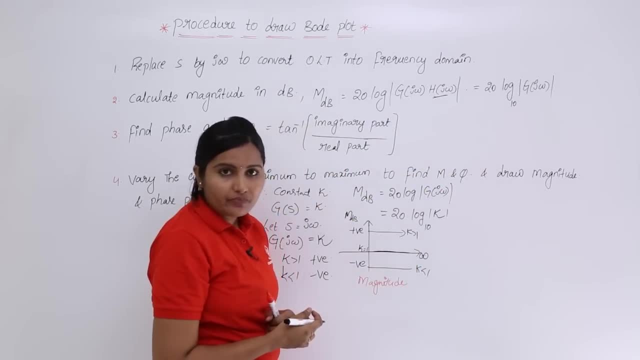 means you need to calculate the phase angle. Phi is equivalent to tan inverse, imaginary part by real part. So here we are not calculating the phase angle. So here we are not calculating the phase angle. So here we are not having any imaginary part. So you are getting tan inverse. 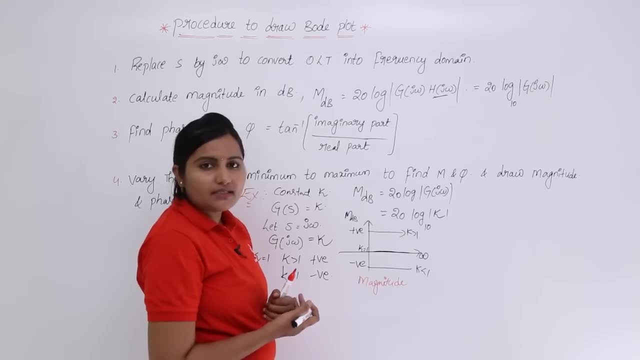 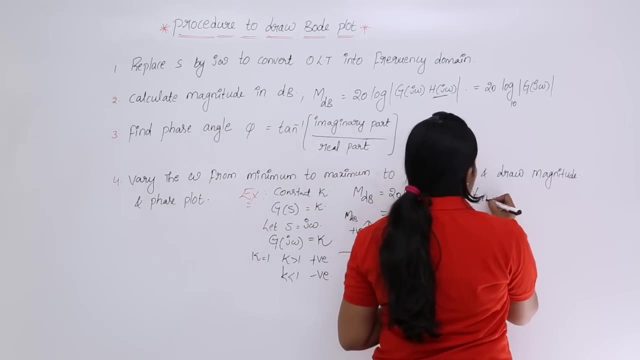 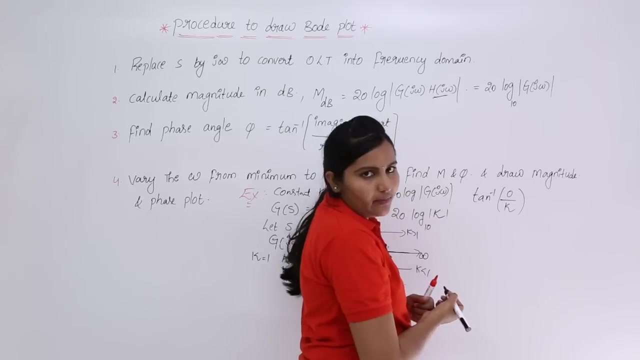 0.. Tan inverse 0 means it is equivalent to 0.. Your phi is equivalent to 0. So here I am considering tan inverse 0 by. So real part is k. Phi is equivalent to tan inverse 0 by k. 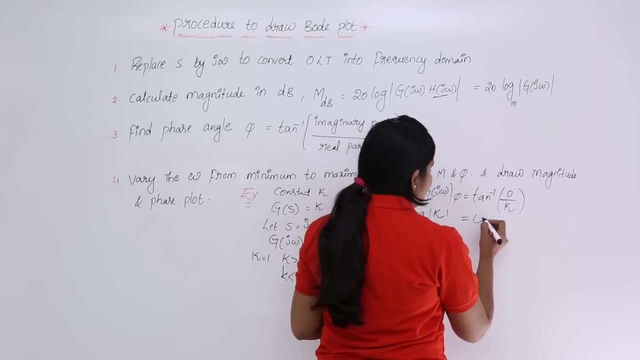 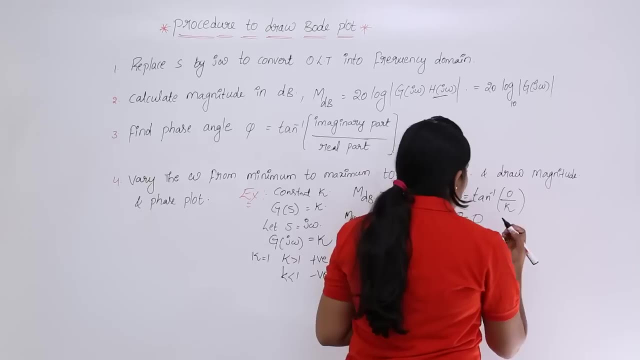 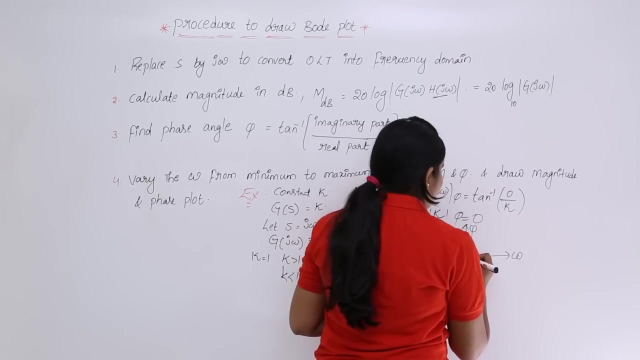 When you are getting tan inverse 0 means when phi is equivalent, You are getting 0.. Tan inverse 0 by k. So now here the phase plot, is So omega. and if you consider phi, So here the phase plot, phi is equivalent to 0. You are not having any plot. 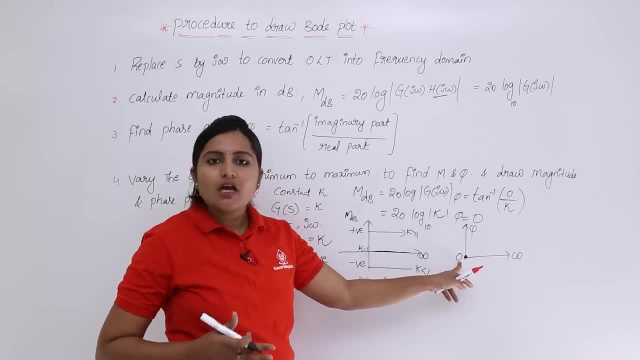 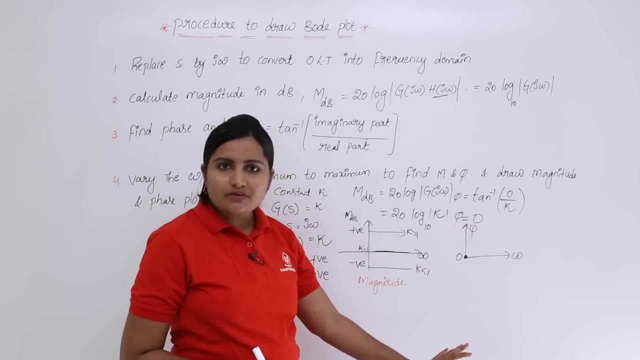 here Your phi is equivalent to 0. Your phase of constant term always will be equivalent to 0.. By combining these two plots you are going to get Bode plot, For example, how we can apply these plots for gate like technical exams means they. 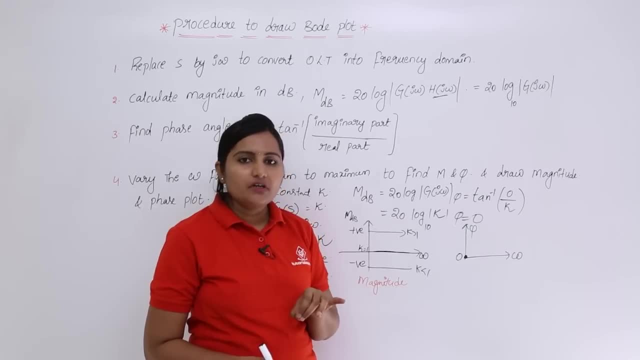 are asking: what is the Bode plot for open loop transfer function equivalent to 2.. G of s is equivalent to 2.. If they are asking like that, then so definitely 2 is a positive value. 2 is greater than 1 value. So we will not get tan inverse 0 by k. So here we are not calculating. 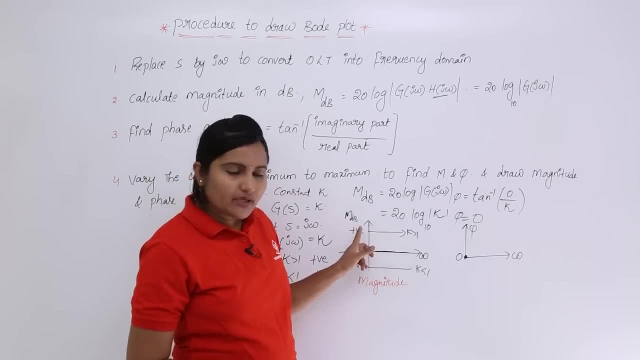 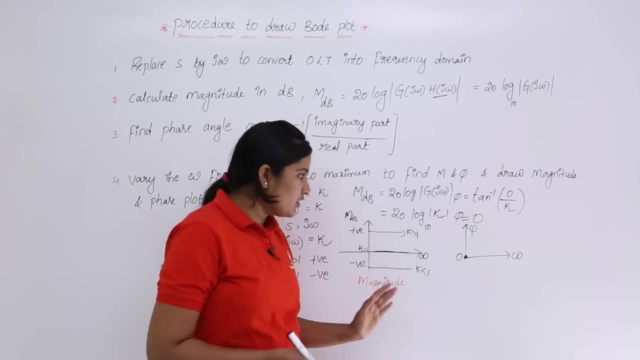 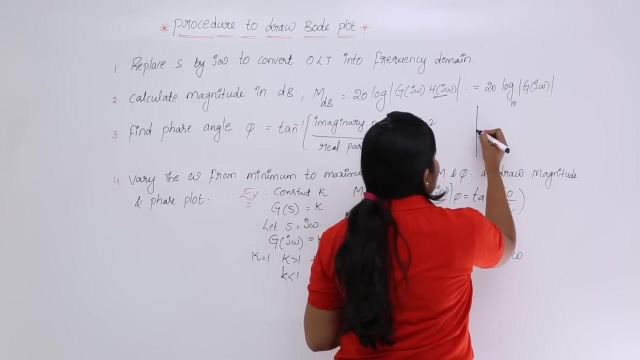 this line. So above omega axis, that means in positive magnitude axis, you will get a line and in phase plot. So generally your Bode plot will be combination of, for example, k is equivalent to 2.. So k equivalent to 2 will be like this. So this is m, This is. 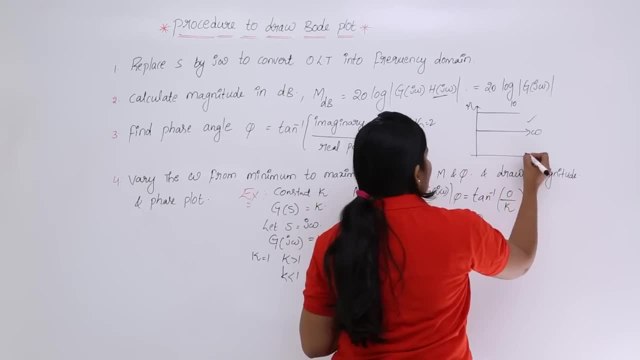 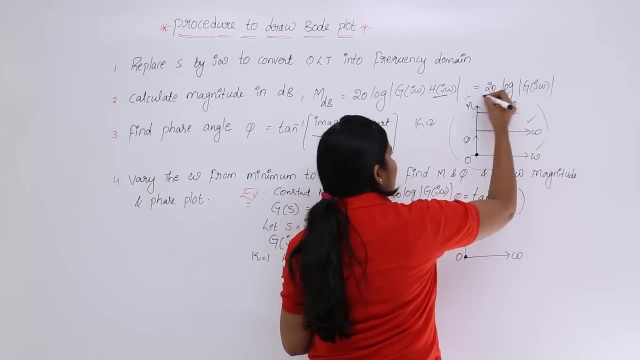 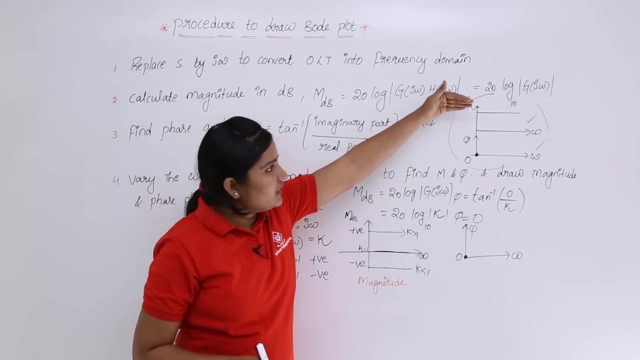 magnitude plot up to here and coming to phase plot. So here also we are going to consider omega and this is phase plot. So this is total Bode plot, for k is equivalent to 2.. For example, if they given k is equivalent to minus 2, then this line will come here. So like that we need